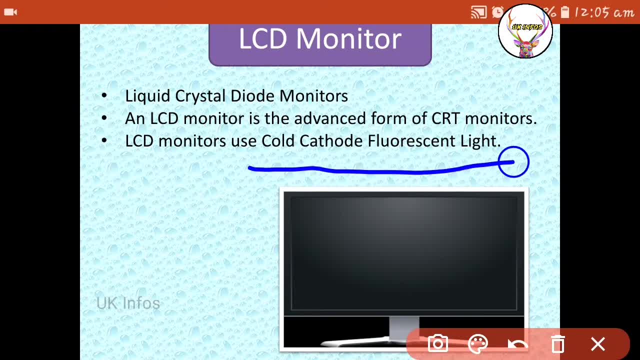 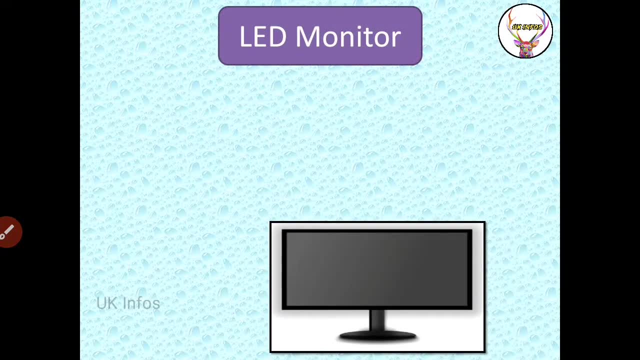 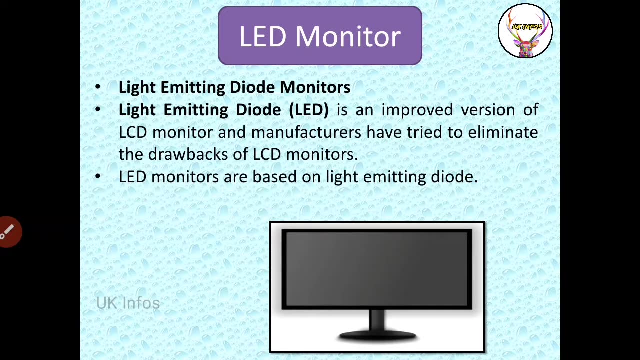 So it is used. cold cathode fluorescent light LED monitor. This is called LED monitor. LED stands for light emitting diode monitors. LED is an improved version of LCD monitor. Manufacturers have tried to eliminate the drawbacks of LCD monitors, So this is one of the advanced levels of LCD. 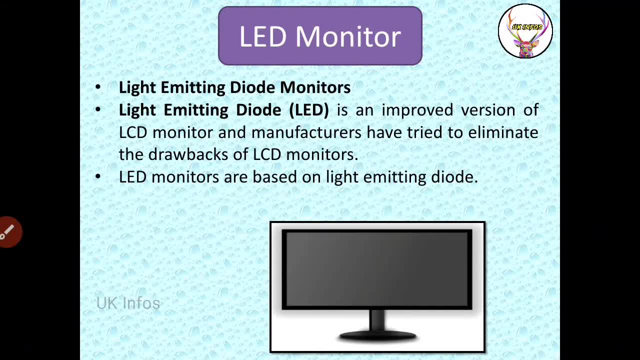 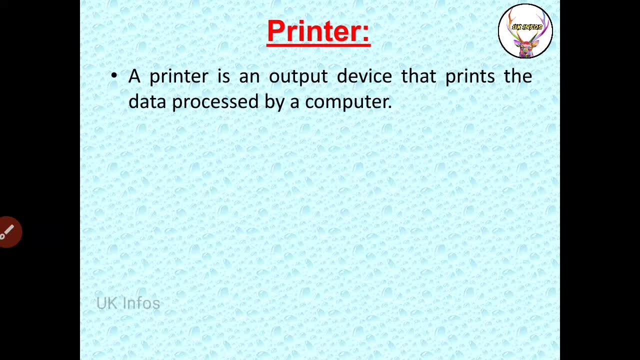 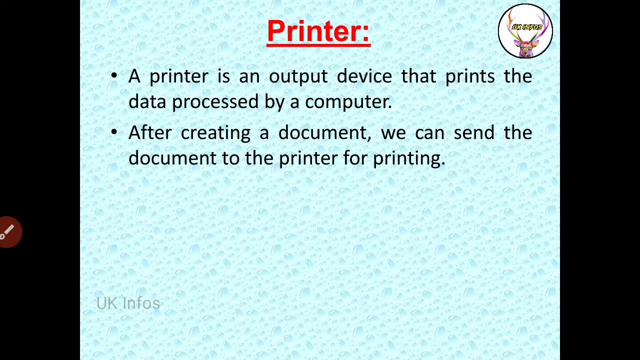 LCD monitors are based on light emitting diode Printer. A printer is an output device that prints data to answer questions about light energy, data processed by a computer. after creating a document, we can send the document to the printer for printing. the printer generates the hard copy known as. 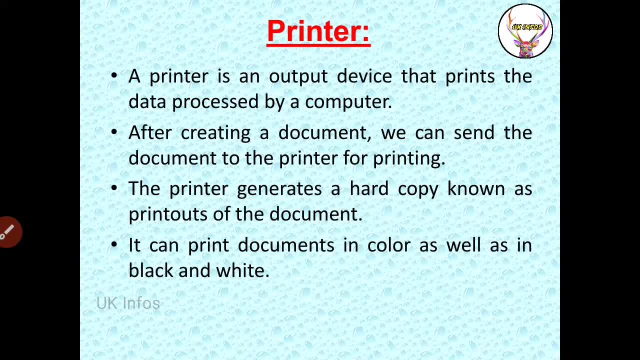 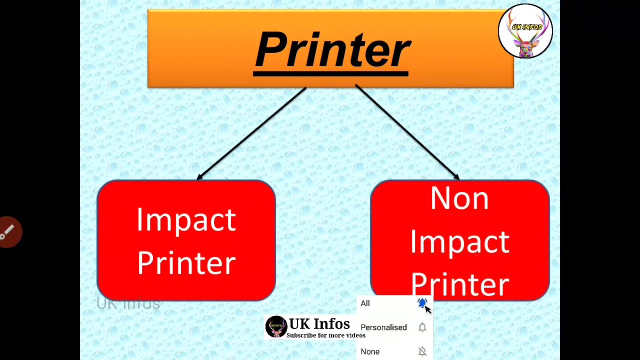 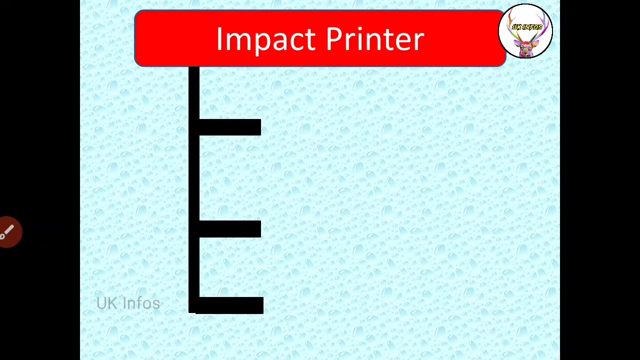 printouts of the document. it can print documents in color as well as in black and white. printers can be classified into the following two categories. the first one is impact printer. the second one is non impact printer. impact printer- impact printer also classify into three types: line printer, drum printer, dot. 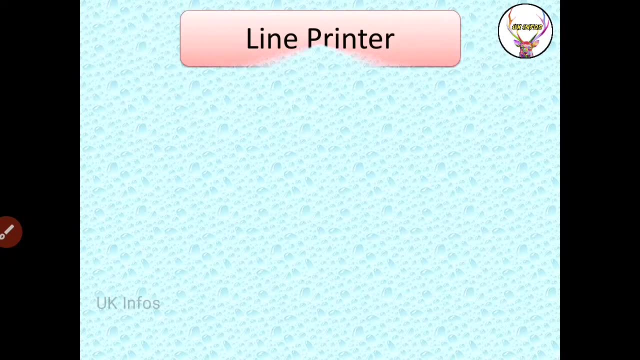 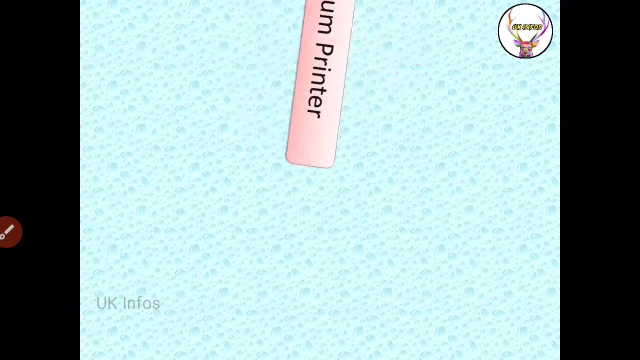 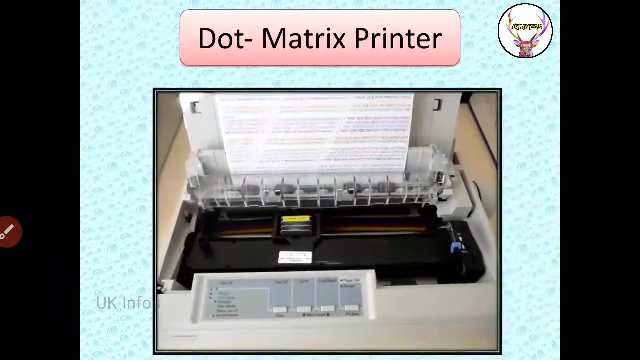 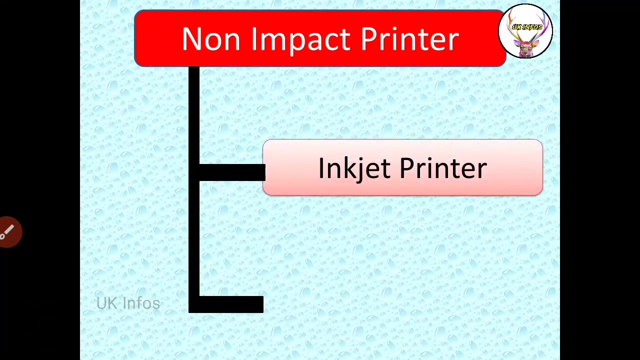 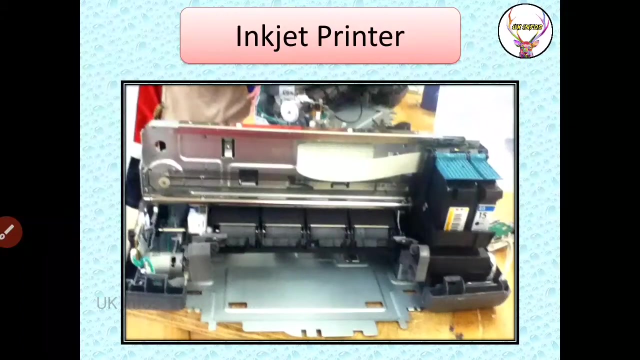 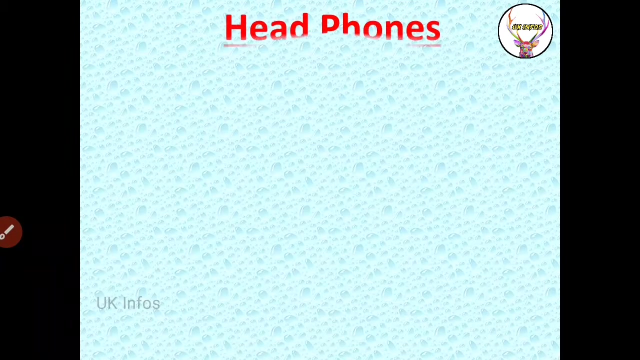 matrix printer, line printer- this is called line printer. drum printer: this is drum printer printer. at last, dot matrix printer. so this is dot matrix printer. non impact printer: the first one, inject printer and laser printer. this is called inject printer, this is called laser printer. next example for output devices: 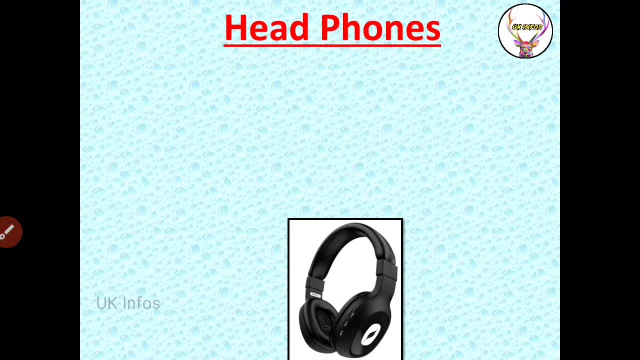 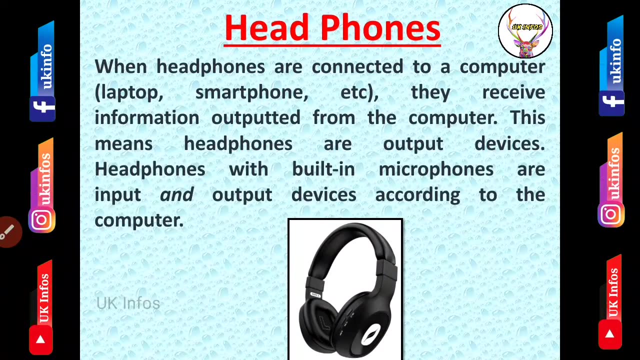 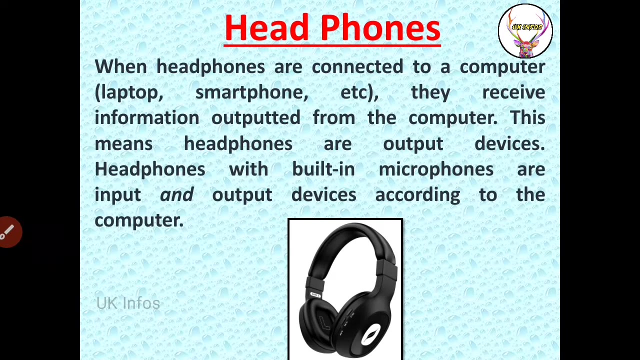 headphone. This is called headphones. When headphones are connected to a computer or laptop or smartphone, they receive information outputted from the computer or the device. This means headphones are output devices. Headphones with built-in microphones are input and output devices according to the computer. 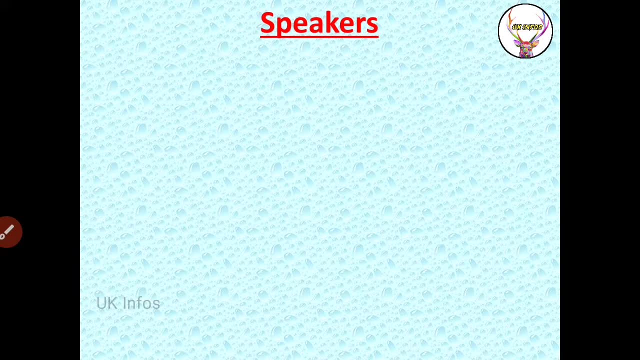 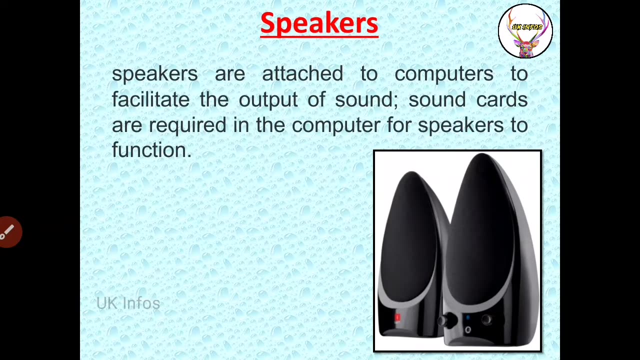 Next example is speakers. This is called speakers. Speakers are attached to your computer to facilitate the output of sound. Sound card is very important, So sound card are required in the computer for speakers to function. So without sound card we could not hear. This is called sound card. 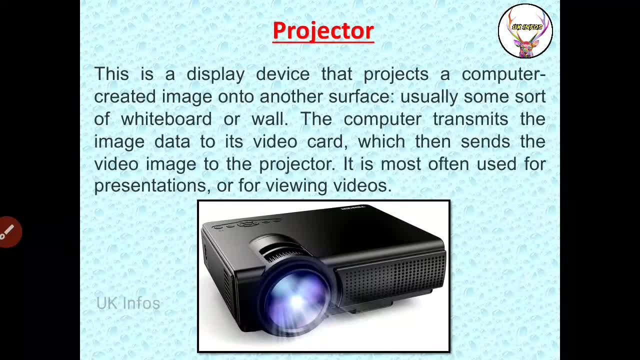 This is a projector. This is a display device that projects a computer created image onto another surface, Usually some sort of whiteboard or wall. The computer transmits the image data to its video card, which then sends the video image to the projector. It most often used for presentations or for viewing videos. 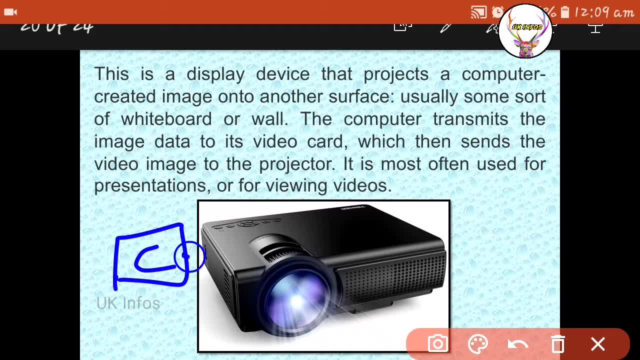 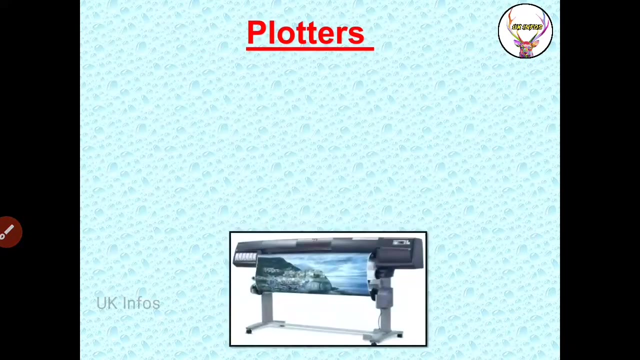 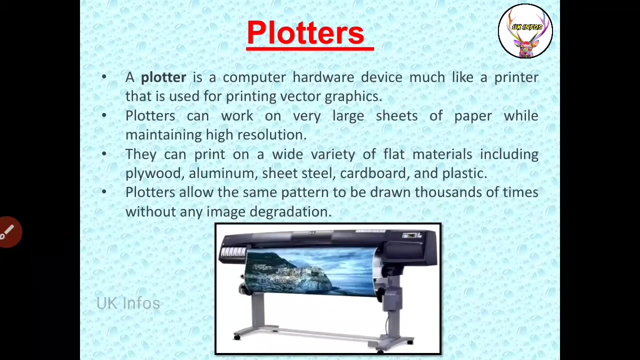 Okay, this is a computer. So computer Transfer the image to the video card and it's sent to the projector. So without video card we could not watch the videos. Plotters- Another example for output device is plotters. This is called plotters. A plotter is a computer hard drive. This is called a computer hard drive. This is called a computer hard drive. 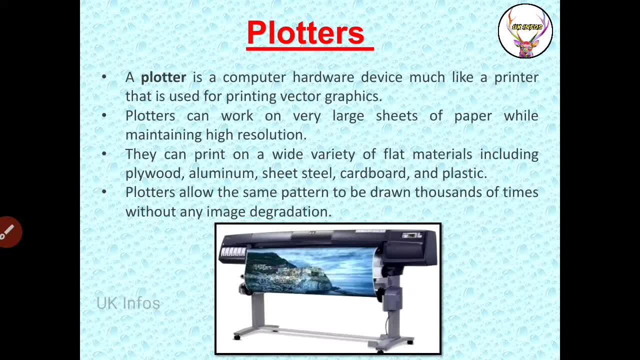 And plotters are 나왔ive device, much like a printer that is used for printing with the graphics. plotters can work on very large seats of paper while maintaining high resolution. They can print on a wide variety of flat materials, including plywood, Aluminium, sheet, steel, cardboard and a plastic. plotters allow the same patentCO. 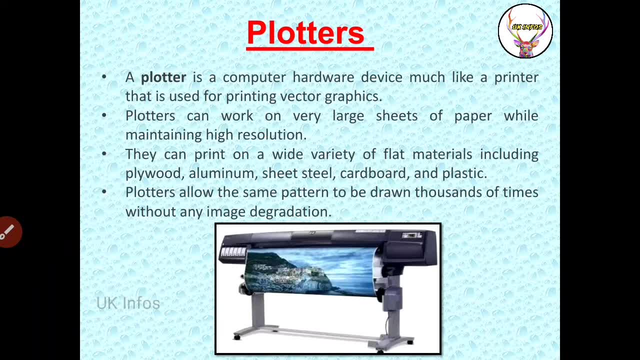 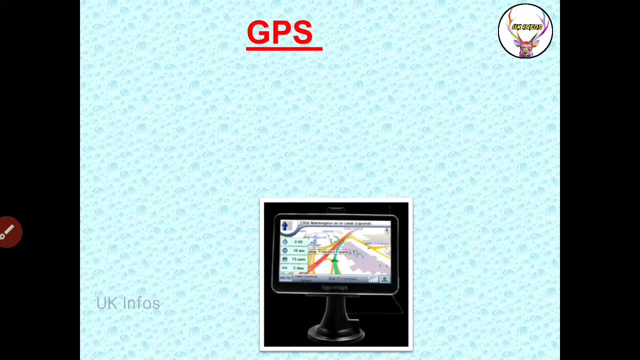 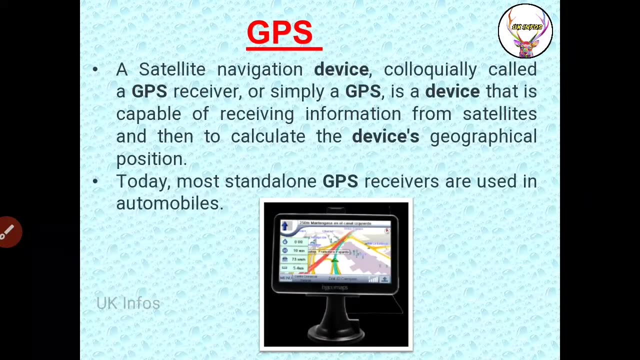 Plotters allow the same patent. We had drowns of tens of thousand of times without any image degradation. so last one is GPS. this is called GPS: we can find out the routes. a satellite navigation device, colloquially called as GPS receiver or simply a GPS, is a device. 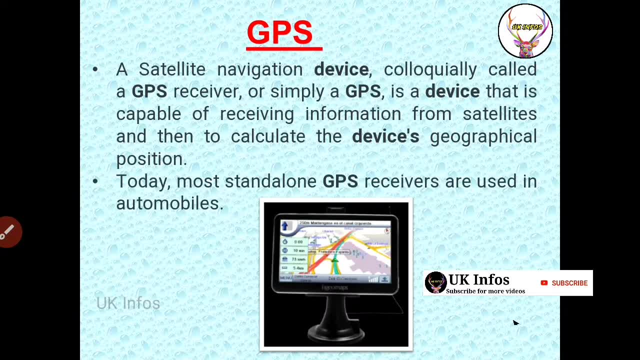 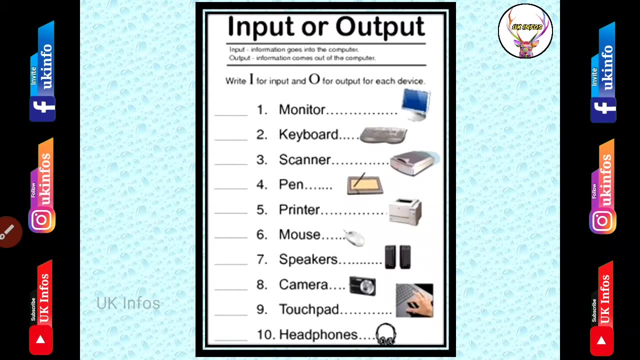 that is capable of receiving information from the satellites and then to calculate the devices geographical position. today, most standalone GPS receivers are used in automobiles. this is a worksheet you can try it out. thank you for watching.